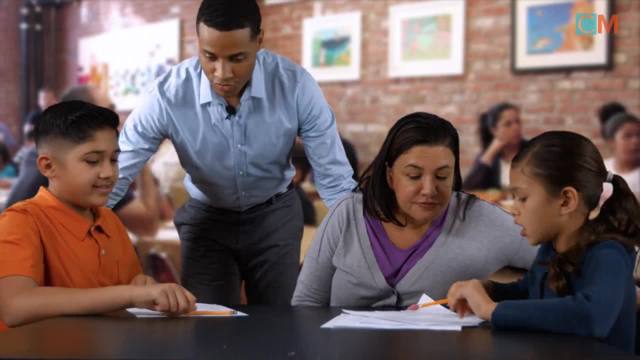 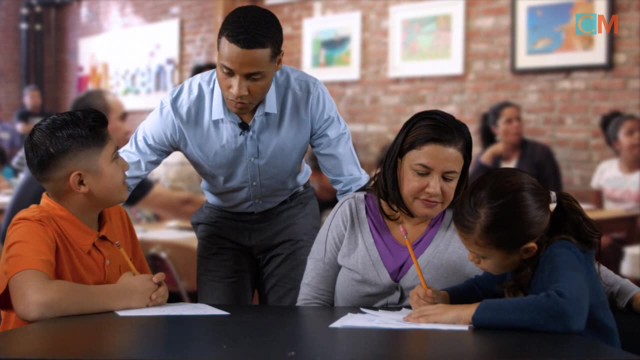 inspire you, So you already know your lines. I'm going to tell you all the things to be able to draw. You already have a really great plan, but let's try adding a little more detail. Okay, so what do you suggest? Let's try adding some arrows to show which direction your prototype will move. 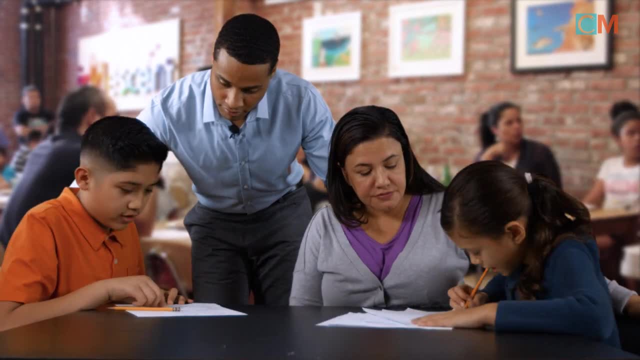 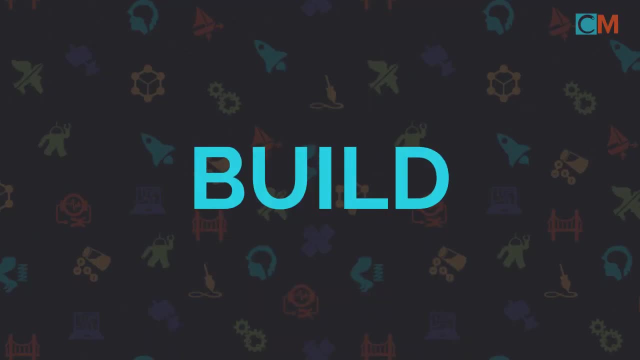 Okay, so I have the cup pointing to the straw and the straw to the balloon and the balloon to the paperclip. Once the plan is ready, it's time to build. Sometimes children have trouble following their plan and they get discouraged. 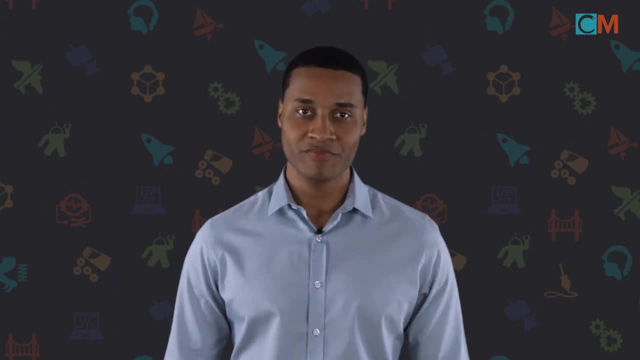 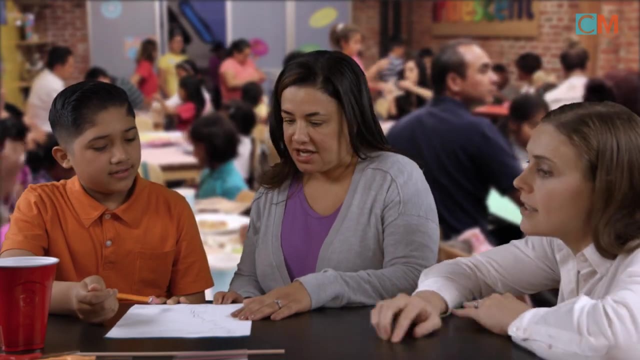 with building. Try sitting down with them and start building together. Involve the family as much as possible to encourage the child. Mom, can you get started? Let's take a look at the plan and figure out what the first step should be. 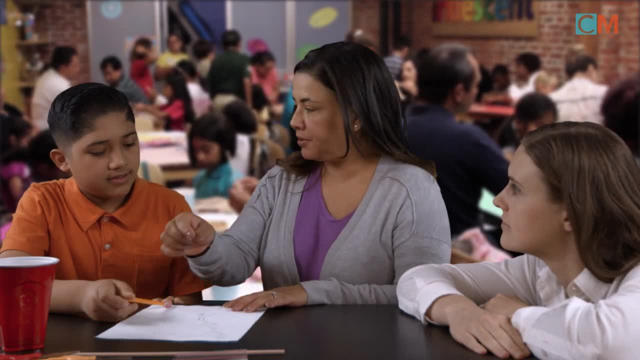 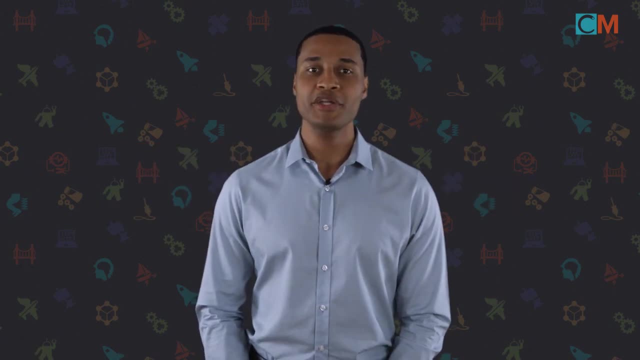 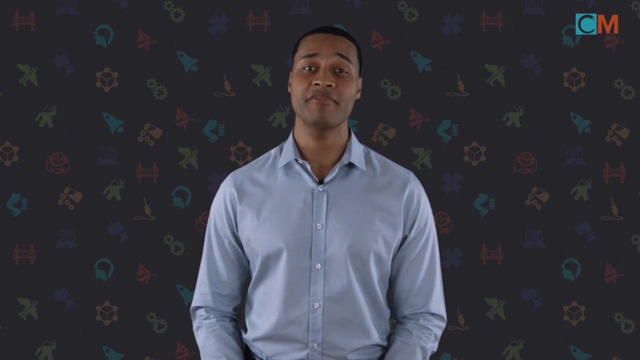 Maybe using the cup Testing will help prove whether or not your design was successful. Make sure you have a spacious testing station for children and their parents. It's important that the child takes note of the problems that their prototype faces when tested, just like you learned. 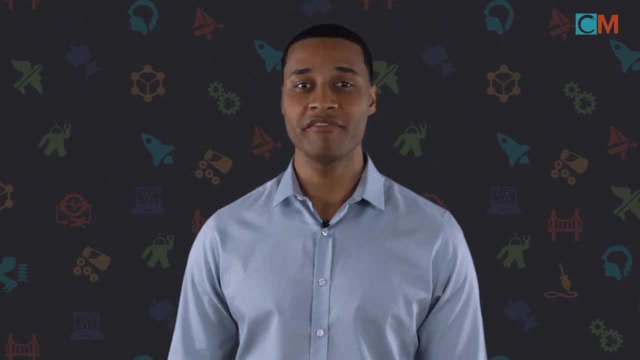 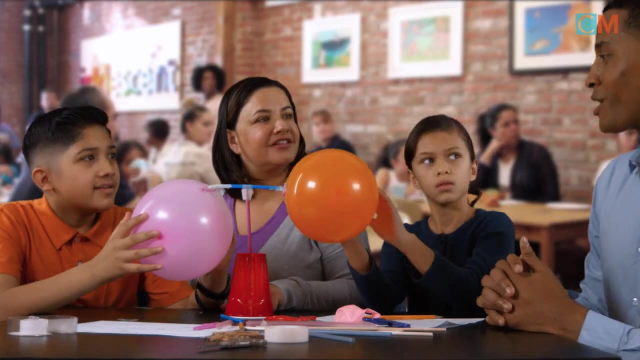 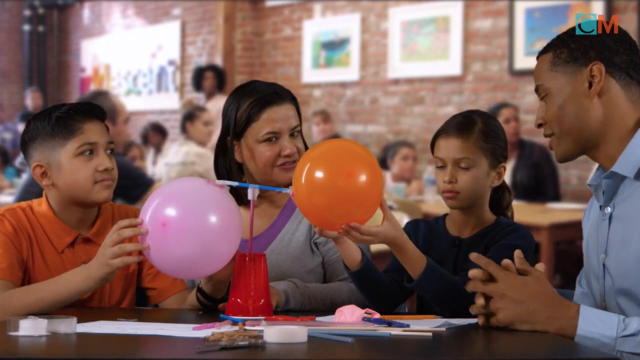 from the errors in your own work In order to make the child aware of the importance of testing stage. try asking questions before testing their design. What do you think is going to happen when we test the prototype? I think it'll spin. How do you think it'll spin? In what direction? 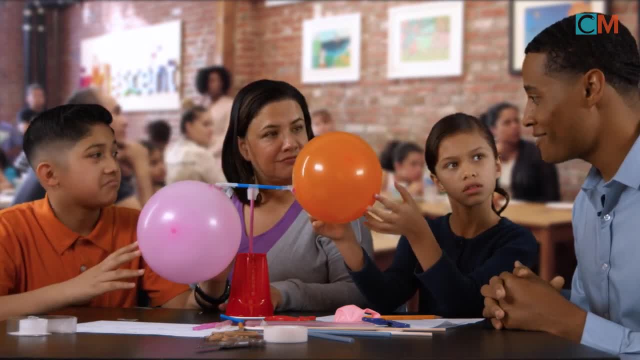 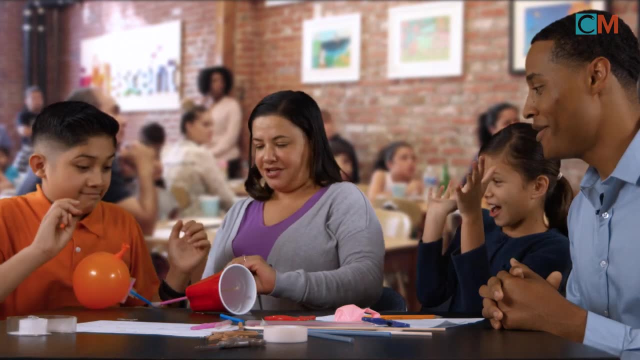 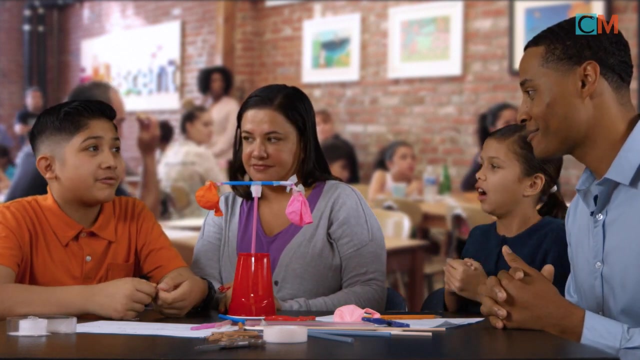 Maybe this way. Well, let's try it out and see Ready One, two, three. So what did we learn from the test? I learned that it needs a stronger supporting structure. It's tilting to the side. What do you think we can do to modify the design to maybe help it spin a little better? 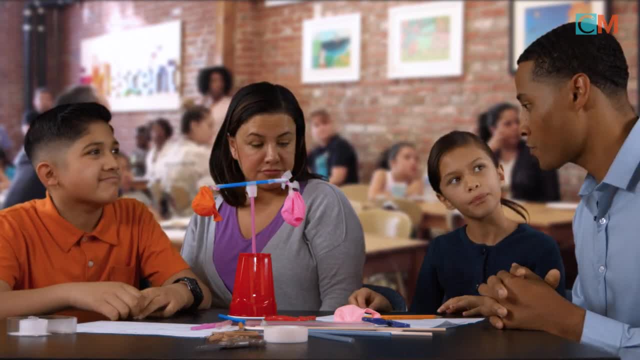 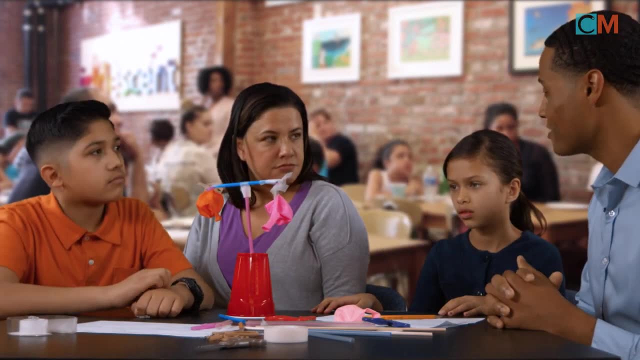 I think we could take the cup to the table. What do you think would happen if we turned one of the balloons in the opposite direction? Do you think that would help it spin? more or less More probably. Well, let's try it out and see what happens.